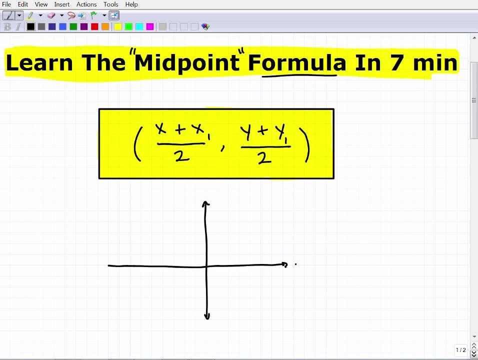 X, Y plane And, if I didn't mention it, this is actually the midpoint formula. Okay, so, this is the midpoint formula, But I'm going to go ahead and explain to you what this is. So let's plot some points here. Let's say this is the point two, two. And let's say this is three, four, five, one, two, three, four, five, six. Let's say this is the point five, six. Okay so, 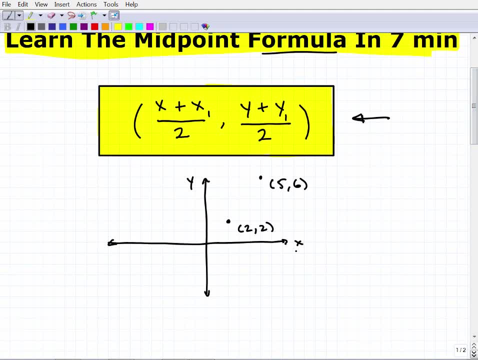 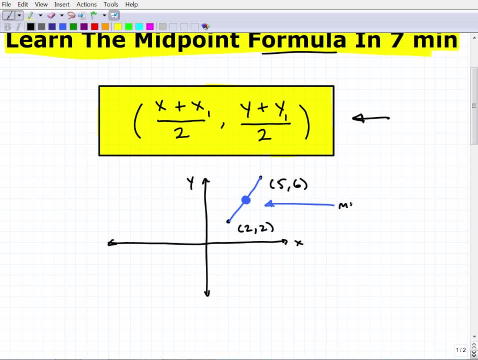 midpoint, here the midpoint, let me just write this here- the midpoint between these two points: 5, 6,. all right, so we got 5, 6 and 2, 2, is this coordinate right there? okay, So the midpoint formula basically is a formula that helps us determine. hey, what exactly is the midpoint? Where's the location of the midpoint? 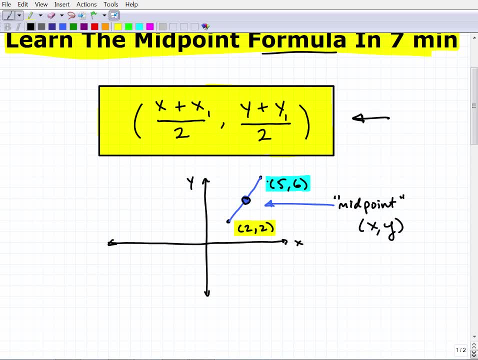 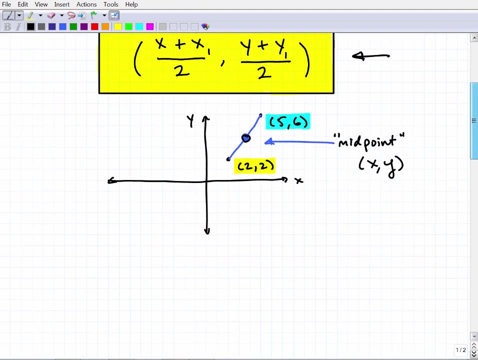 point, the mid point in between these two points. so this is what we're doing and it's actually a very easy formula to apply. okay, so what we're looking at here in terms of the midpoint form is simply another way of stating taking the average of the two points. so the midpoint, if 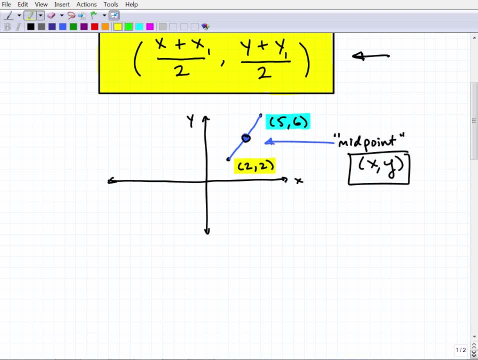 you can agree with me is going to be some x- y point. right, that's a point. so it's going to have an x and a y, all right. so you say, okay, yeah, I get that. so the midpoint will have an x and a y. now the x value is going to be the average of the x's, okay, the x's that are involved here. so 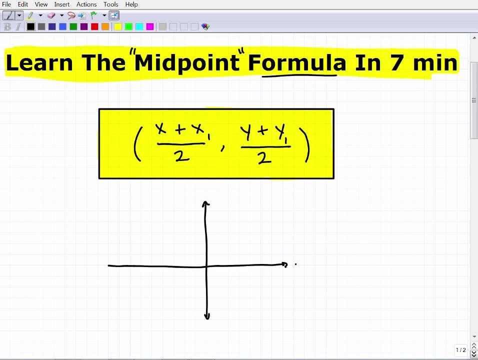 X, Y plane And, if I didn't mention it, this is actually the midpoint formula. Okay, so, this is the midpoint formula, But I'm going to go ahead and explain to you what this is. So let's plot some points here. Let's say this is the point two, two. And let's say this is three, four, five, one, two, three, four, five, six. Let's say this is the point five, six. Okay so, 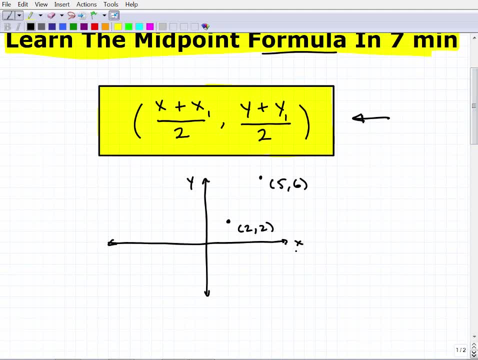 I have two points on the X- Y plane. Okay, now what I want to do. let's just think of a line that goes through, a line that connects these two points. Okay now, somewhere along this line is the midpoint, ie. 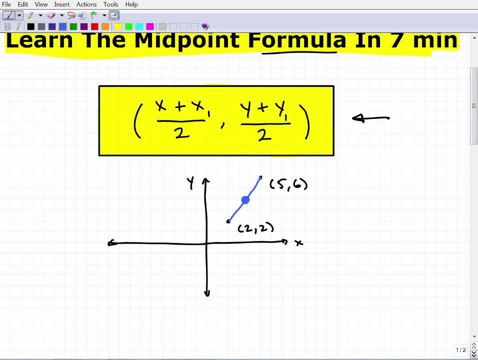 the middle way between these two lines, right Like right there, more or less. Well, this is what we call the midpoint. So the midpoint here and the midpoint- let me just write this here- the midpoint between these two points. five, six, all right. so we got five, six and two, two. is this coordinate right? 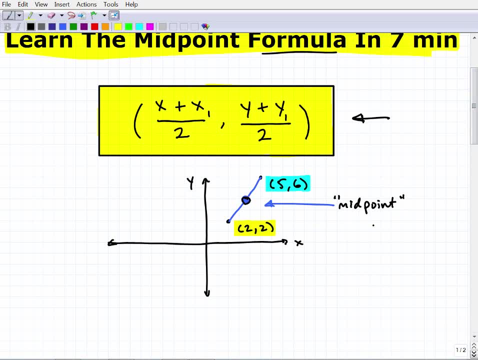 there, okay. so the midpoint formula, basically, is a formula that helps us determine: hey, what? what exactly is the midpoint? where is the location of the midpoint, the midpoint in between these two points? so this is what we're doing, and it's actually a very easy formula to apply, okay, so what we're looking at here, 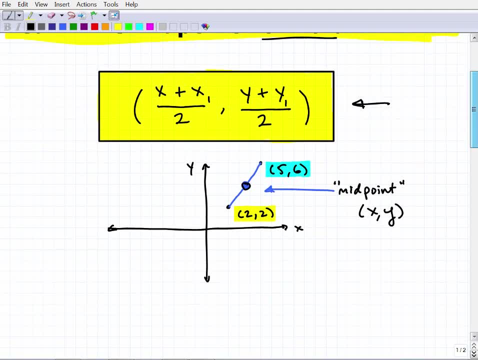 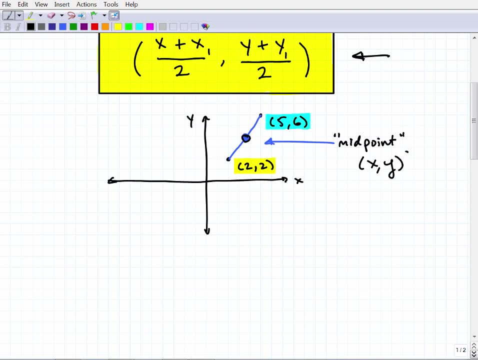 in terms of the midpoint, form is simply another way of stating taking the average of the two points. so the midpoint, if you can agree with me, it's going to be some XY point. right, that's a point. so it's going to have an X and a Y. 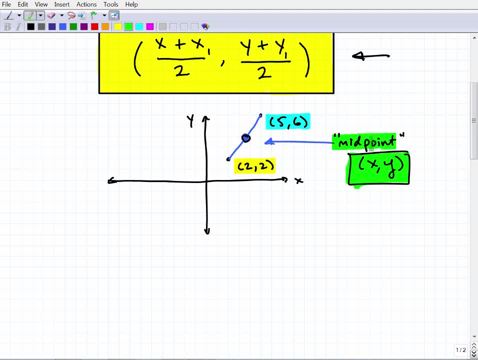 all right, so it's okay. yeah, I get that. so the midpoint will have an X and a Y. now the X value is going to be the average of the X's- okay, the X's that were involved here. so the this two and this five are the X's right. these are the X's. the 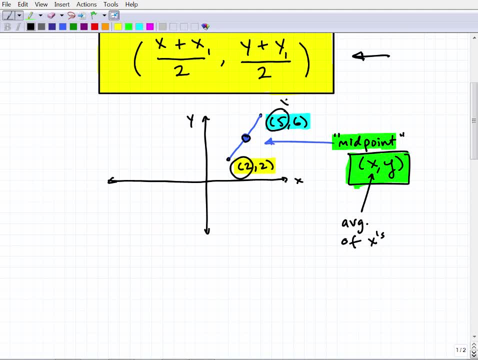 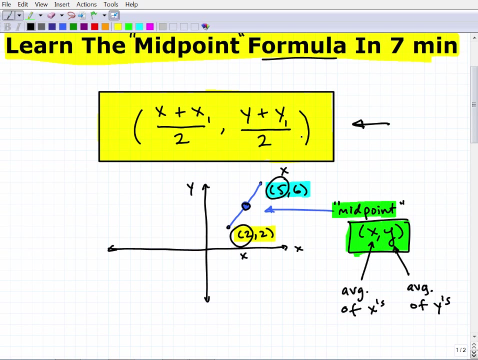 the this two and this five are the x's. right, these are the x's. the first number in order pair are the x's, and the y value here of the midpoint is going to be the average of the two points of the y's. okay, this is what this formula means. okay, how do we find the average? well, we're going. 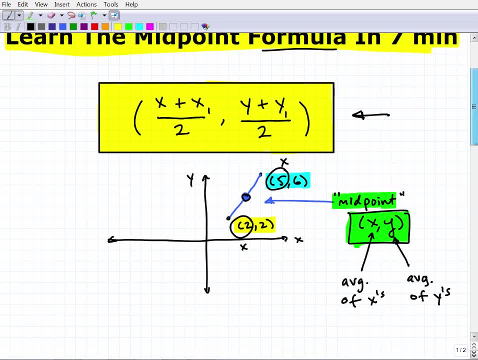 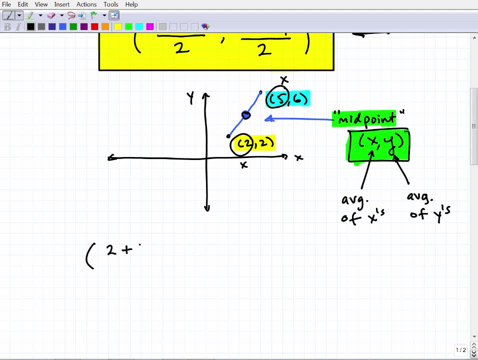 to add up the two points and divide by two. okay, very simple. so let's go ahead and actually apply that here. so the midpoint is going to be two plus five. two plus five over two. okay, that's going to be our x coordinate, and then our y is going to be two plus six over two. so that's going to be. 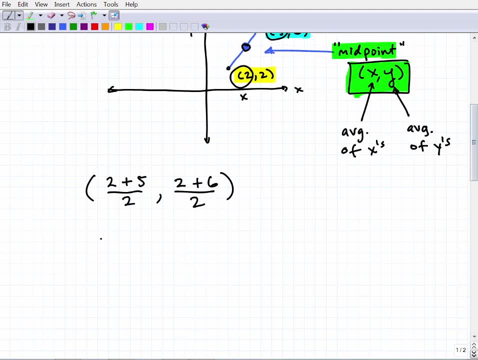 seven over two, all right, so let's go ahead and figure that out. so we're going to get the point seven over two, comma eight over two, and of course we can simplify this further. this is seven halves divided by eight over two. is what four, right? so if you want to, you could turn the um the seven over. 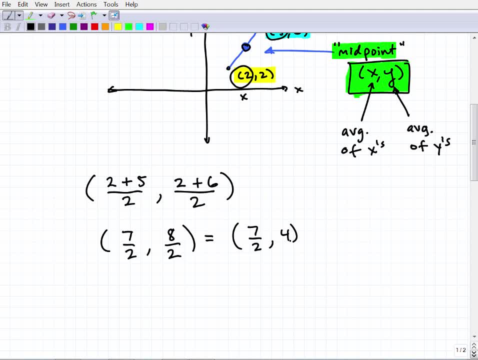 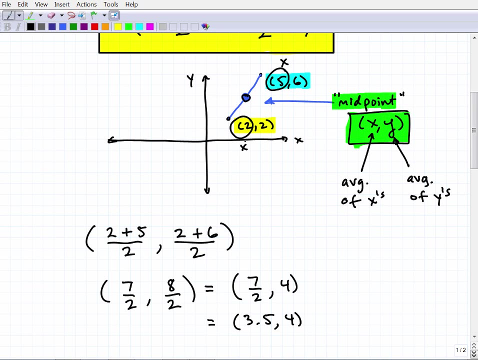 two into a mixed number, but let me just go ahead and give it to you as a decimal. seven divided by two is three point five. right, it's three and a half. so here we have three point five comma four. so let's see- uh, you know this was a sketch, but let's see if this kind of makes sense here in our 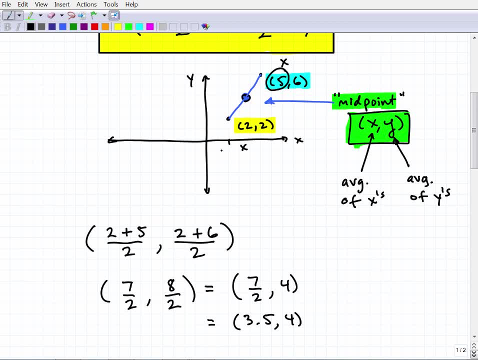 little diagram. so this three point five. well, this is two, right, one, two. here's three and then here, if you kind of notice, it's about 3.5. okay, so that makes sense. now let's see if it's around four. so this is one, two. 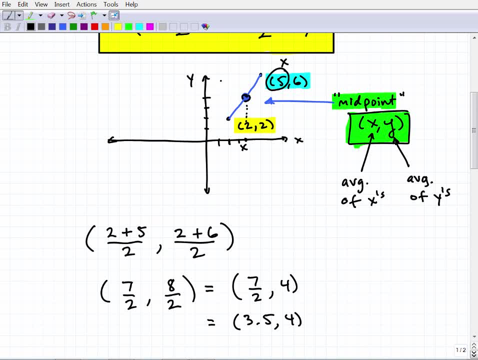 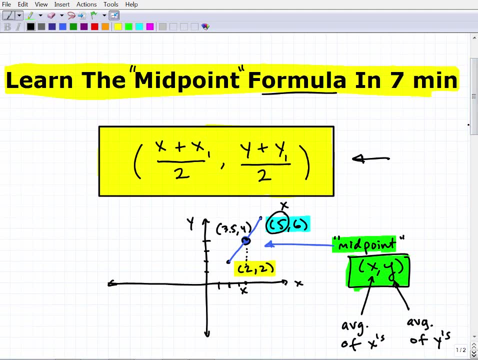 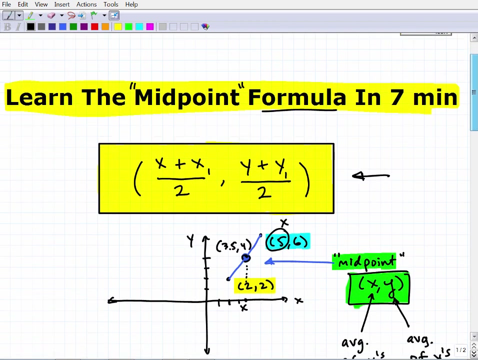 two, three, four, perfect. okay, so this is three point five comma. four is the midpoint. so pretty straightforward stuff. um, the midpoint formula is often taught with the distance formula, so I also have another video on that. actually, I have several videos on, uh, the distance formula and other topics as well, so but let's go ahead and call this a wrap. um, I don't know if I am early or 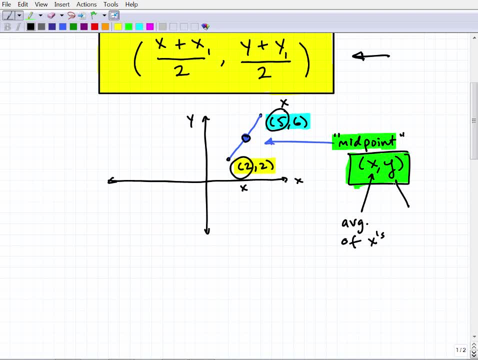 first number in order pair are the X's and the Y value here of the midpoint is going to be the average of the Y's. okay, this is what this formula means. okay, how do we find the average? well, we're going to add up the two points and 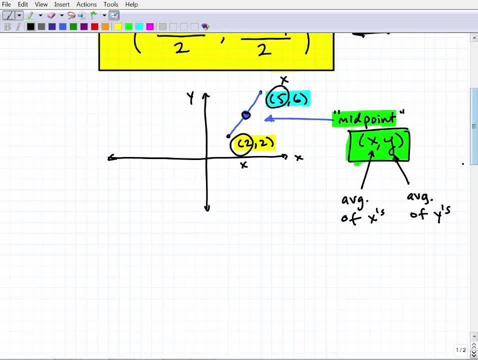 divide it by two. okay, very simple. so let's go ahead, actually apply that here. so the midpoint is going to be 2 plus 5,, 2 plus 5, over 2, okay, that's going to be our X coordinate, and then our Y is going to be 2 plus 6 over 2. alright, so 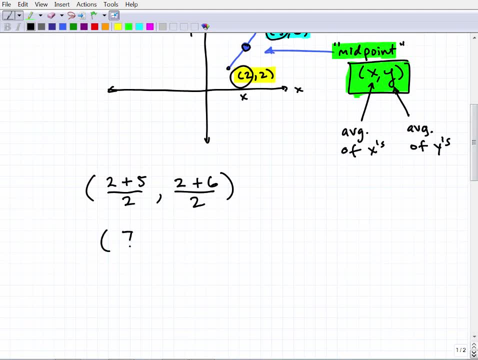 So let's go ahead and figure that out. So we're going to get the point 7 over 2, comma 8 over 2.. And of course we can simplify this further. This is 7 halves divided by 8 over 2, is what. 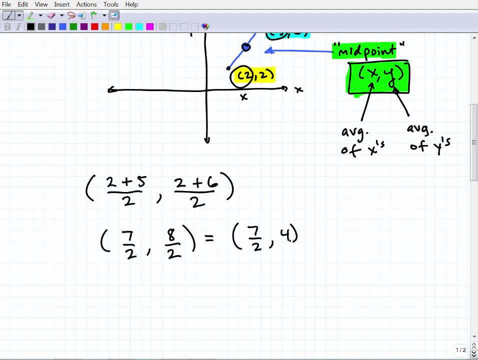 4, right. So if you want to, you can turn the 7 over 2 into a mixed number, But let me just go ahead and give it to you as a decimal: 7 divided by 2 is 3.5, right. 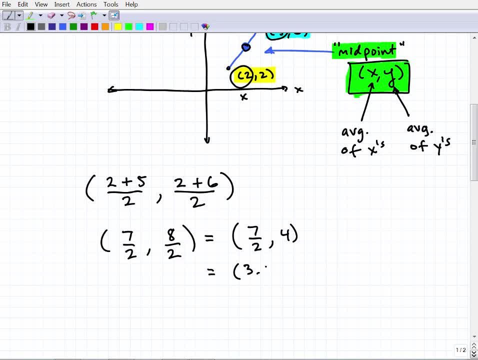 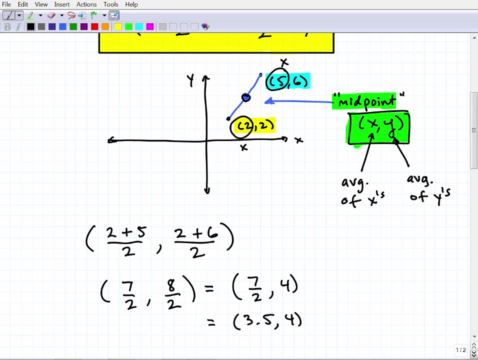 It's 3.5.. So here we have 3.5 comma 4.. So let's see- You know this was a sketch, But let's see if this kind of makes sense here in our little diagram. So this 3.5, well, this is 2, right. 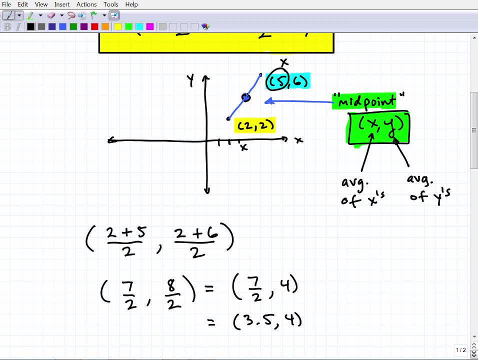 1, 2.. Here's 3.. And then here, if you kind of notice, it's about 3.5.. Okay, so that makes sense. Now let's see if it's around 4.. So this is 1,, 2,, 3,, 4.. 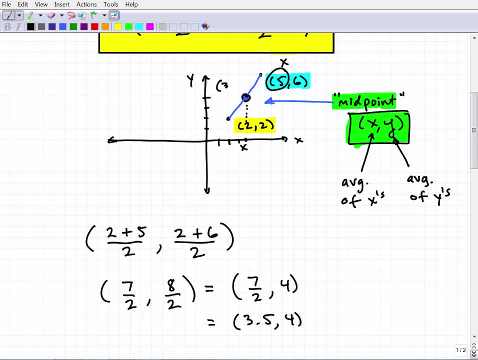 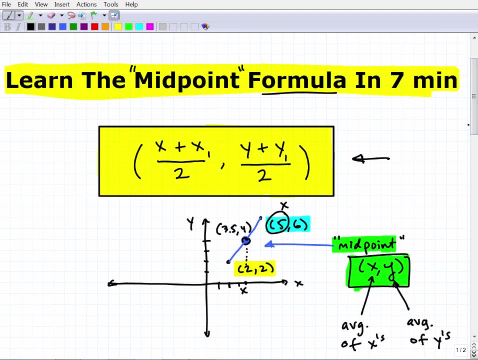 Perfect. Okay, so this is 3.5. comma 4 is the midpoint. So pretty straightforward stuff. The midpoint formula is often taught with the distance formula, So I also have another video on that. Actually, I have several videos on the distance formula and other topics as well. 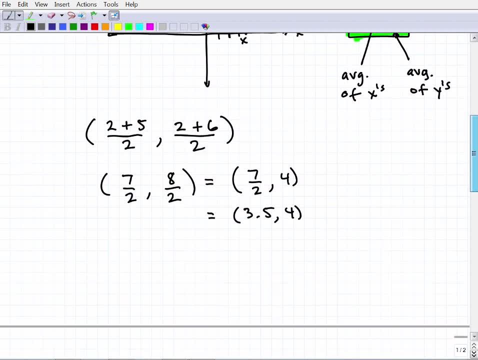 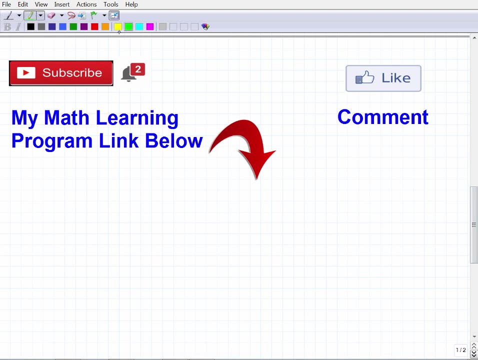 So, but let's go ahead and call this a wrap. I don't know if I am early or late. I try to be. I think I'm getting. I think I'm pretty close to the seven minutes, but we'll see when I finish.